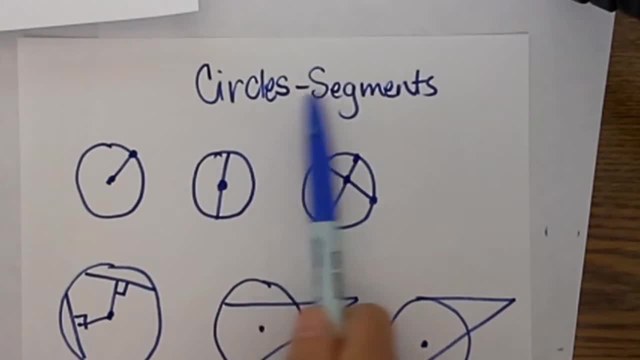 Hi, welcome to MooMooMath. Today we are going to look at segments associated with circles. We have several segments associated with circles. The first segment that everyone should be familiar with is from the center to the edge. that is a radius. The second segment goes all the way through. 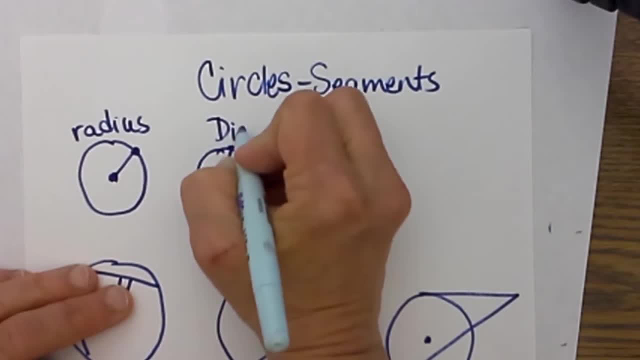 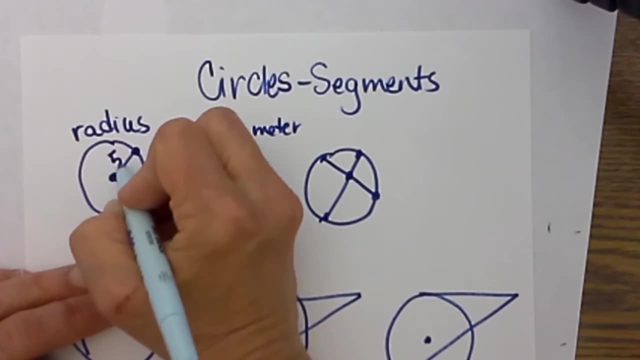 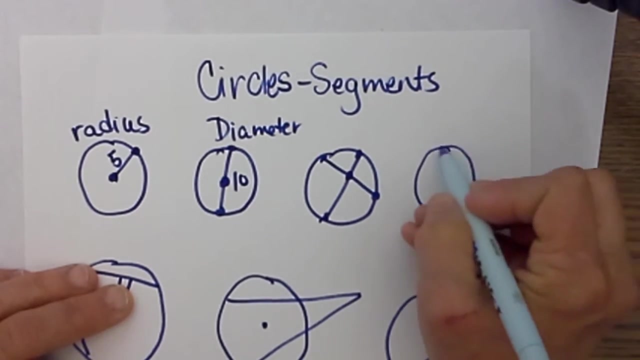 the center of the circle, and that is a diameter. The radius to diameter is a 1 to 2 ratio, so if the radius is 5, the diameter would be 10.. It is twice the length. You also have a chord. A chord is just a segment whose end points lie in the circle, but it 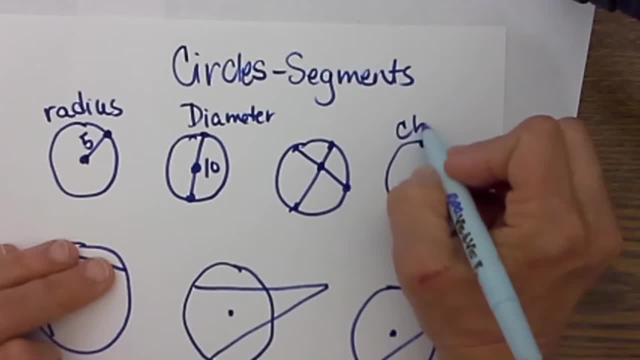 doesn't go through the center like a diameter. That one is just a chord. Let's look at the second segment. The second segment goes all the way through the center of the circle and that is a diameter. The third segment goes all the way through the. 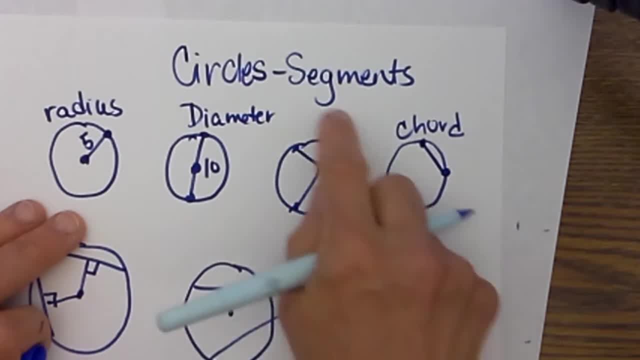 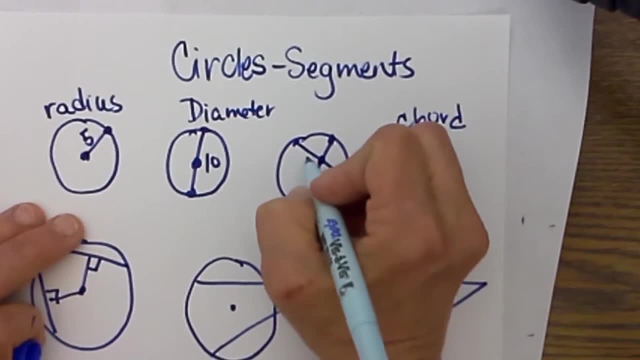 center of the circle. Let's look at a couple situations with chords. Here is the first one. Let's say we have two chords and they intersect. To find one of these links is a cool formula. You take A times B or you take the segment. 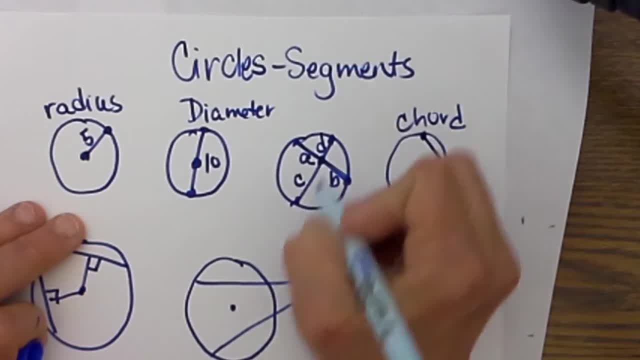 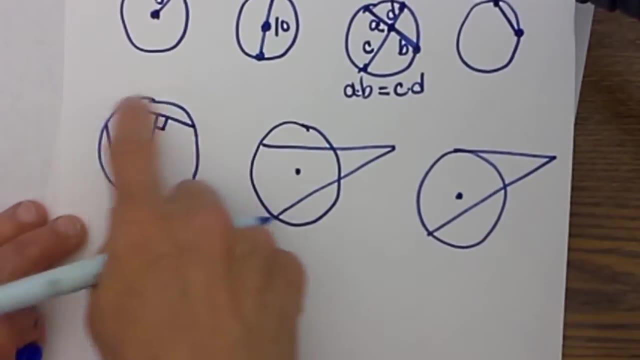 in the two pieces and you find the product. You take one segment: A, B is equal to the product of C times D and that will give you those segments. I will do an example of one of those. Let's say you have a circle and you have two chords. 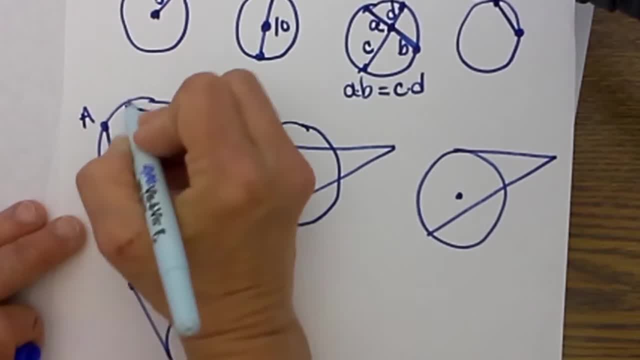 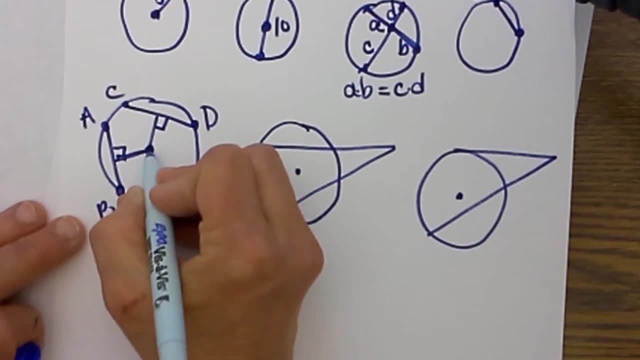 We have a chord here, let's call this chord AB and we will call this other chord CD. If both of these chords are equidistant, so from the center of the circle to that actual chord, if those distances are the same, we have right angles and we also know that it. 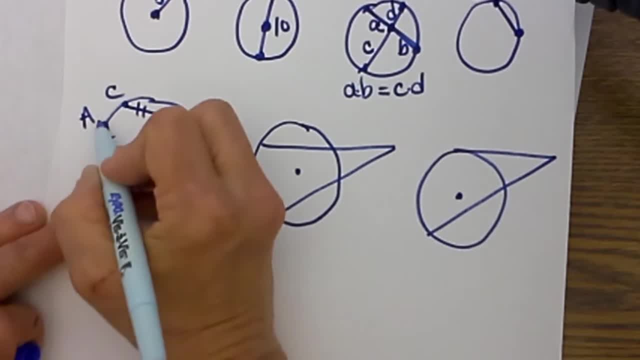 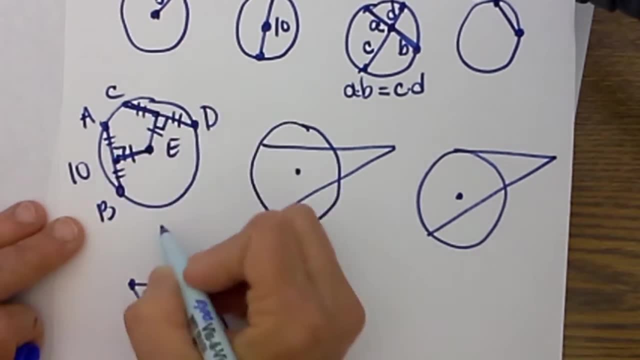 cuts these chords into two congruent parts. So you might know that AB is 10,. well, what is CE? What would this segment be? We know this whole chord would also be 10, so that segment would be 5, and that is how. 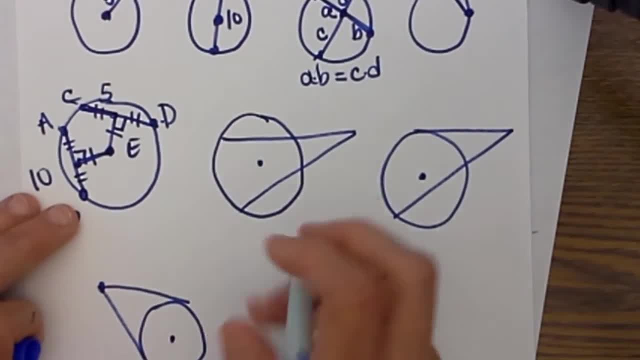 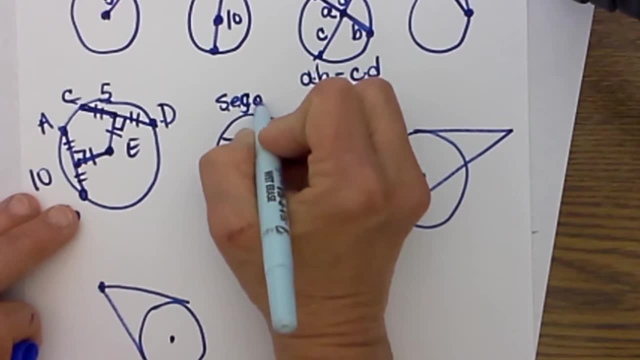 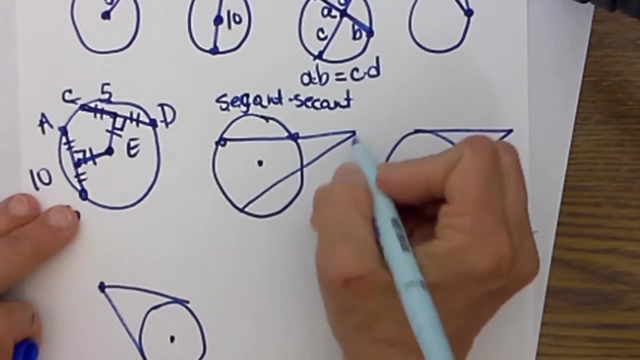 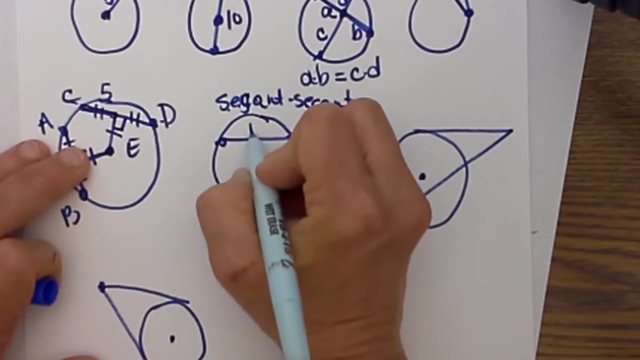 those work. They are pretty simple. The next one would be what we call a secant situation. A secant is a segment that goes through the circle. We have two secants here and we are going to label these parts A, B, C and D. Those 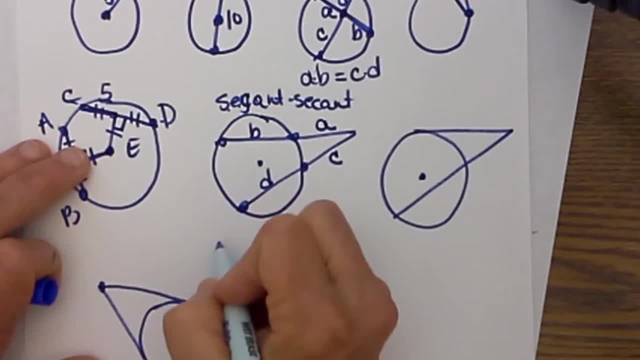 are secant segments, as we call them. So we are going to take A times A plus B and we are going to set that equal to C times C plus D. In other words, you take the exterior segment times the whole segment and the exterior segment times the whole segment and set them equal to U. 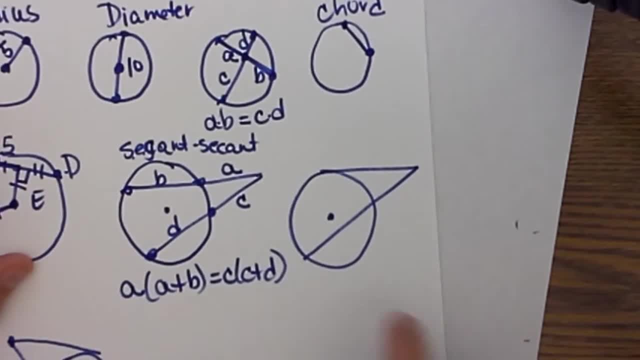 E. We will do a bad example of this in a moment. The next one is a tangent and secant Tangent. secant works similar to a secant secant. I'll call this secant tangent because a tangent is just a line that touches the circle in one place. 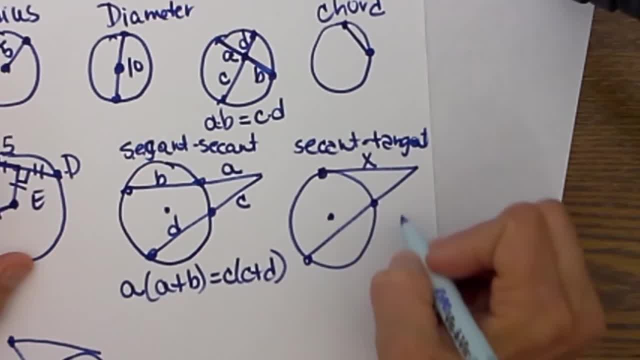 For this segment. we will call this segment X variant AB. So you treat the secant segment just like you did this one. You take the exterior times, the whole thing, so you have A times A plus B, and you set it equal to this tangent squared, so X squared, and that is the formula for that one. 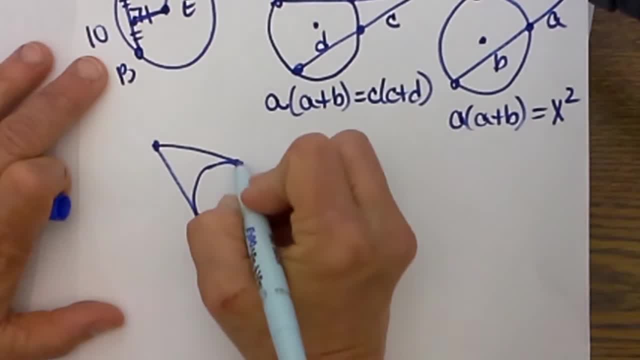 The very last one of these is the tangent. tangent. so you have an exterior point and you draw a line of tangency to the circle on both sides. This one is so simple. these two segments are congruent to each other because they are touching the circle from an exterior point. and then the other nice thing is there is a right angle. 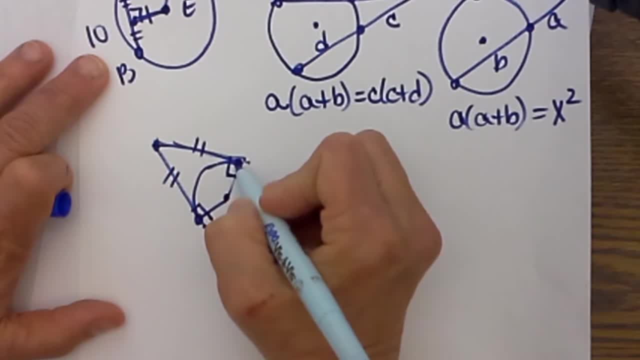 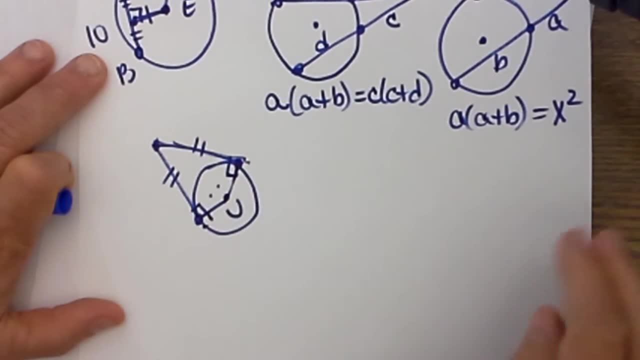 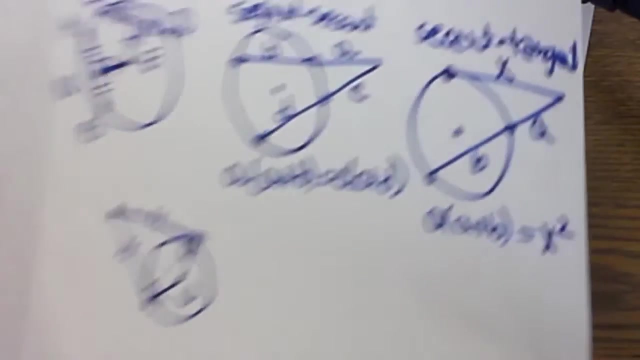 so from the center to the tangent point of tangency, you have right angles and you can do all kinds of cool things with right angles. I also like to call that one the party hat rule. so you can draw a little party hat and you can see the hat would have to be congruent on both sides. 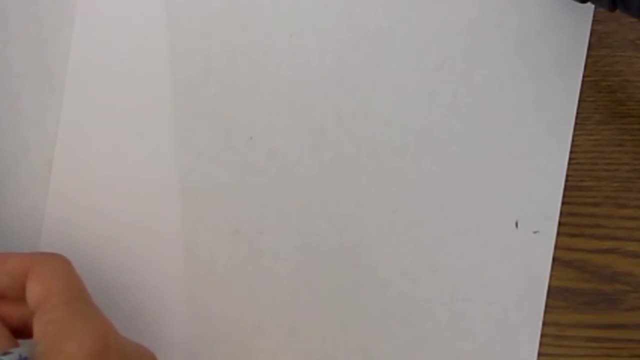 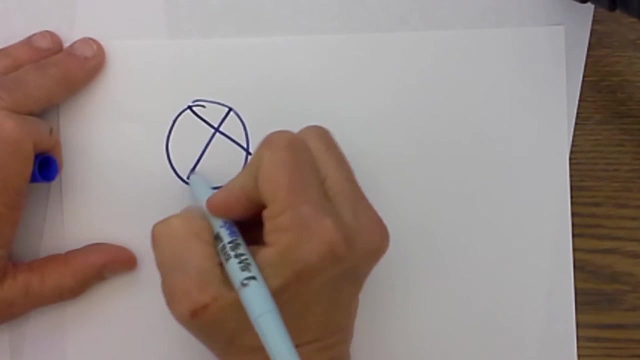 Now let's look at a couple quick examples. Let's do an example of a circle. Let's say this segment is 3, this segment is 4 and this segment is 2, and we don't know this longer- one Based on the chord chord. we will take 2 times X and set it equal to 3 times 4, so we get 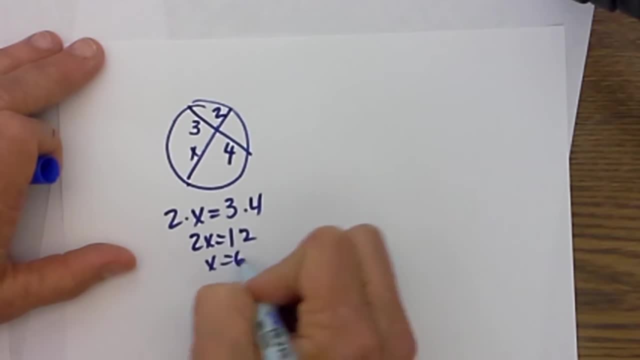 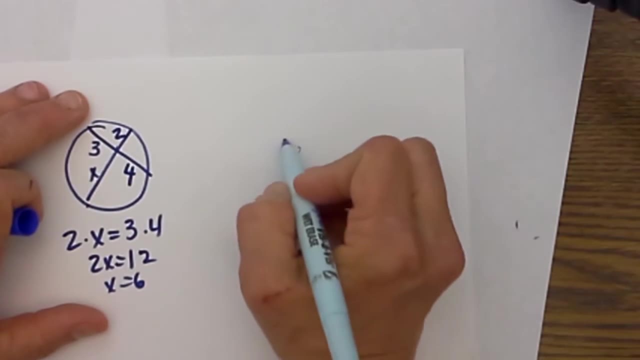 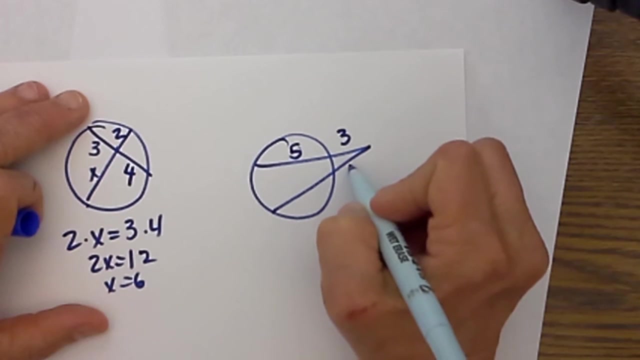 2X is equal to 12 and X is 6.. That means this secant segment is 6.. Now let's look at one that is a secant secant. Let's draw a secant secant. This is 3, this is 5, this is 2 and this is X. 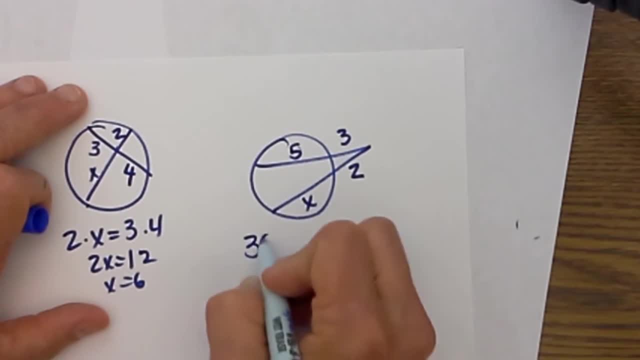 This one we take the outside times, the whole thing. so we will take: 3 times 3 plus 5 equals 2 times X plus 2, so you will add those together to get the whole secant segment. So you will have 3 times 8, which is 24, and X plus 2 equals 4.. 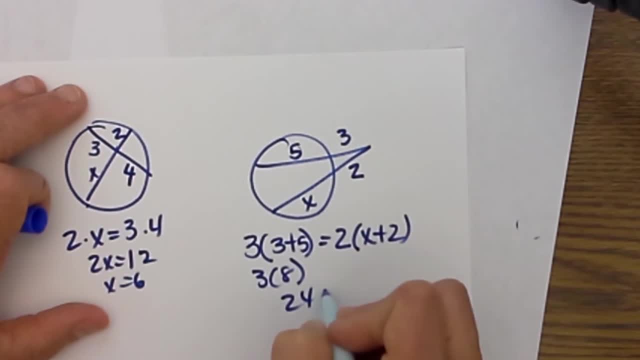 Now let's draw a secant secant. Let's draw a secant secant. Let's draw a secant secant. Let's say: this is 3, this is 5, this is 2 and this is X, and that is equal to 2x plus 4, which is subtract 4 from both sides. so we have 20 equals 2x. 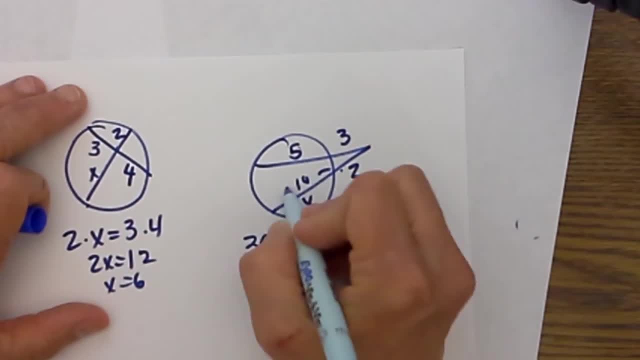 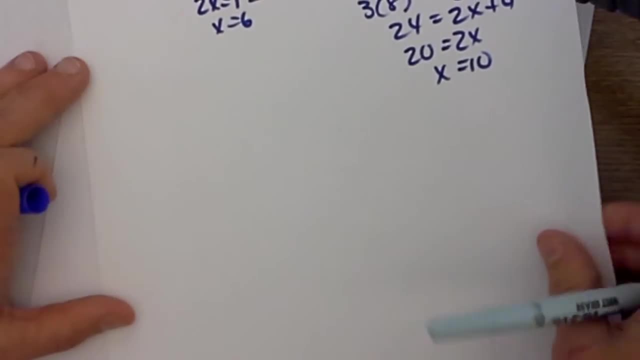 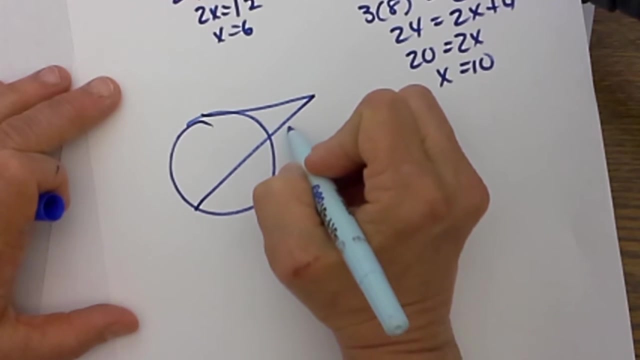 so x is 10.. That means this segment is 10.. So that is how that one works. Now let's look at a secant tangent. So here is our circle and we have a tangent segment and then a secant. Let's say, this is 4 and this is 12, and we don't know our tangent segment. 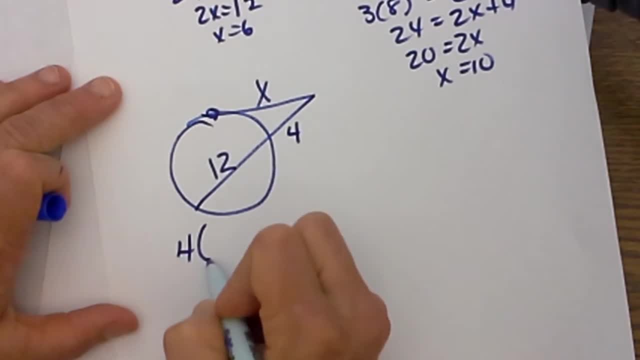 The secant segment. you treat the same. You take 4 times the whole thing, which is 4 plus 12, and that is equal to the tangent segment squared. So we will have 4 times 16, which is x squared, and 4 times 16 is 64, so that means x is equal. 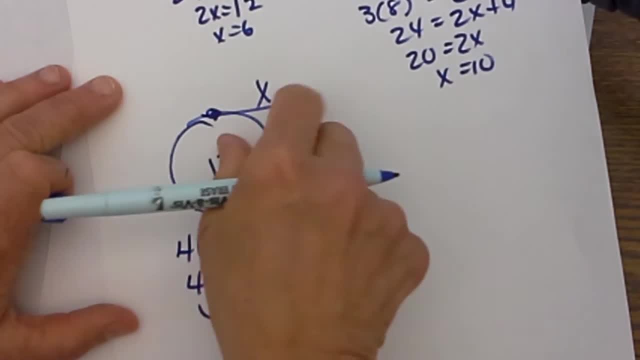 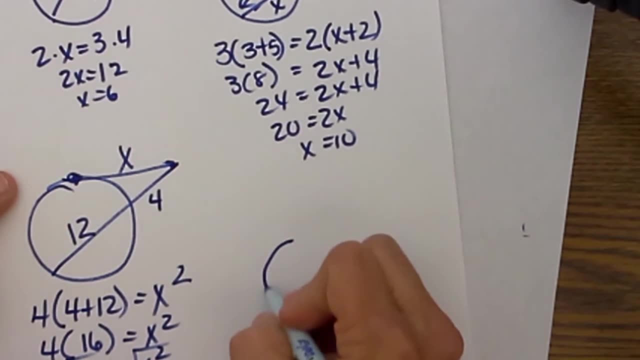 to 8.. It wouldn't be negative 8 because you can't have a segment that is a negative value. So that is a secant tangent. and let's look at a party hat rule. If you have a point out here and let's say you know this is 2x and you know this is 3x.